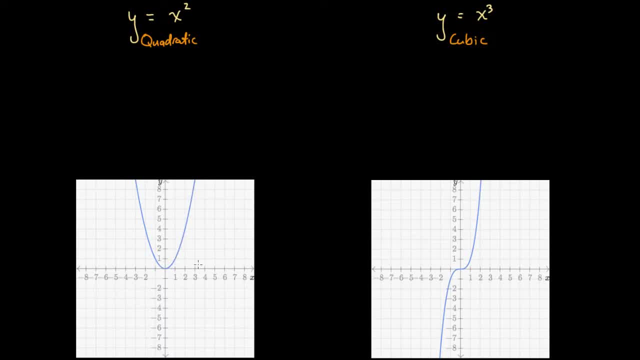 and it seems that the y values are increasing faster than the x values on both sides here, on the right-hand side of the origin. But on the left-hand side we have quite a different story. For this quadratic function we have only positive y values, whereas the y values 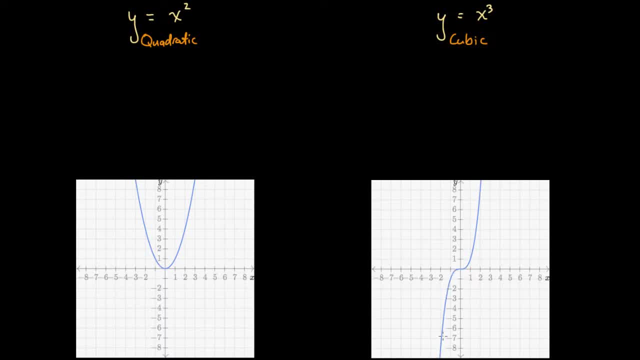 for this cubic function we have negative y values, And we'll examine why that's the case in a moment, why that's a consequence of the algebraic construction of these functions. The other feature we may notice is that on this right-hand side of the graph for all. 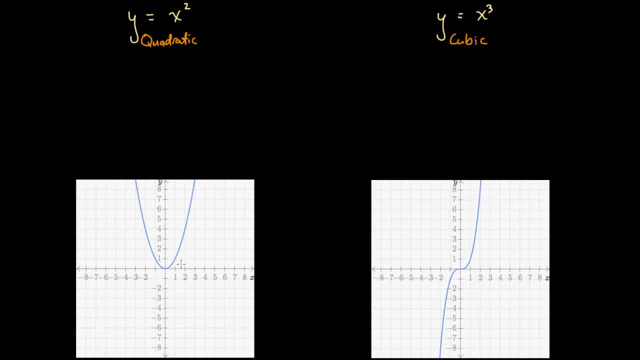 values greater than x equals 1, we have the y values increase at a slower rate than for the cubic function. So, for instance, if we were to do the same thing here, we would have x squared and y squared. If we were to have a look at x equals 2, here we have x equals 2 is associated with. 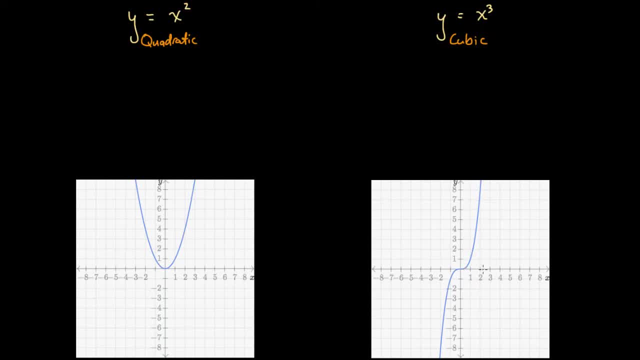 a y value of 4,, whereas in this cubic function we've got x equals 2 is associated with a y value of 8,, which suggests that the y values are increasing after x equals 1 much more rapidly for the cubic function than for the quadratic function. 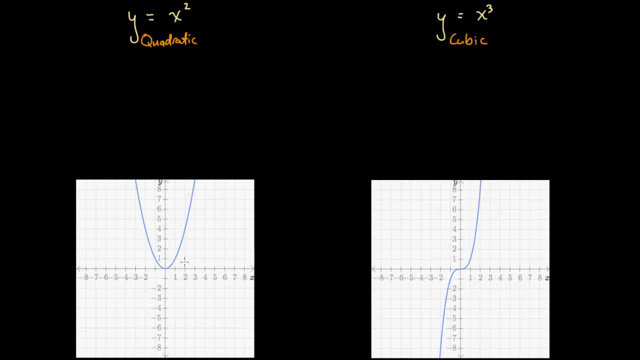 Okay, well, examining that value x equals 2 is actually quite interesting, especially when we evaluate what happens at x equals 2 and at x equals minus 2.. So let's go ahead and just consider those two values. So let's consider that at x equals 2, here we have y equals 2, squared. 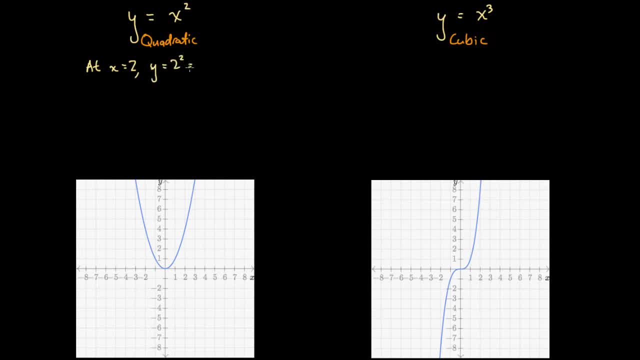 So y equals 2 squared, 2 squared equals 4.. We can go ahead and plot that on our quadratic function here, So 2 units right at the origin and 4 units up. Moreover, when we have x equals minus 2.. 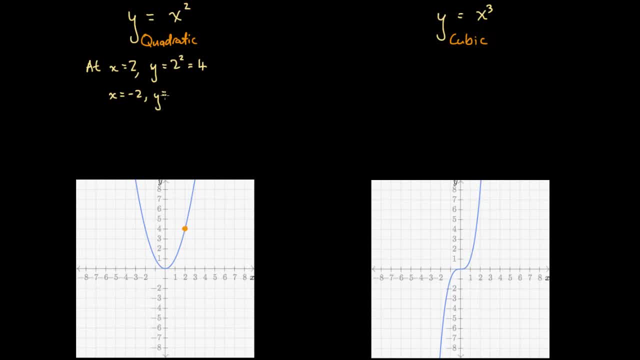 We have: y equals minus 2 squared. Minus 2 squared, a negative times a negative is a positive. so negative 2 squared equals positive 4. We can go ahead and graph this as well, so it's going to be 2 units left of the origin. 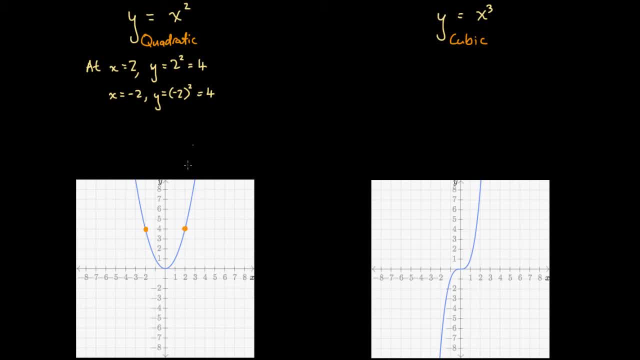 and 4 units up. So we've discovered here that the reason that we have no negative y values associated with this quadratic graph is the property of negative numbers. Now, that is that when you multiply the y values, you get the property of negative numbers. 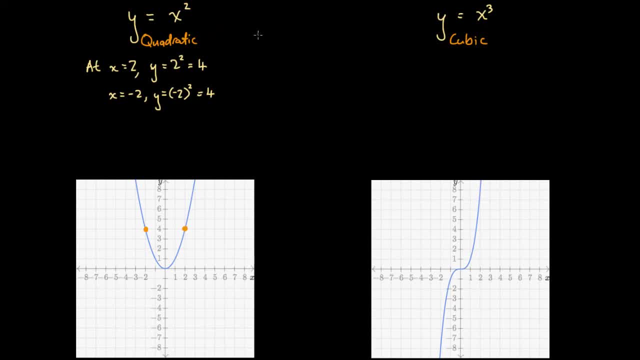 That is, that when you multiply the y values, you get the property of negative numbers. So if you multiply a negative number by a negative number, you always get a positive number. So if you multiply a negative number by a negative number, you always get a positive. 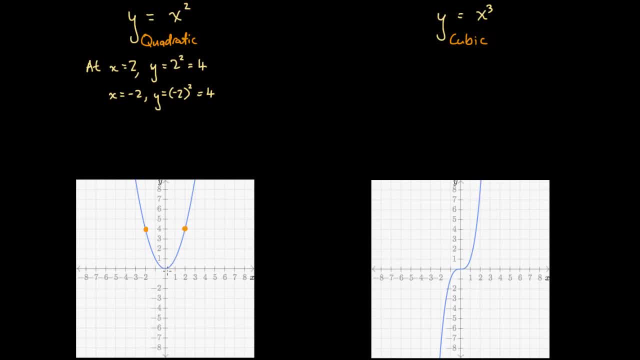 number. Consequently, if we substitute any positive x value or any negative x value into this function, we're always going to get a positive y value. Consequently, all the y values, all the y coordinates of these points are going to be positive. 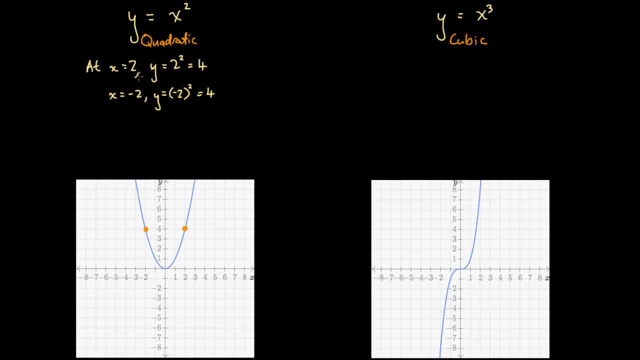 But that's not the case for this cubic function. Let's examine why. Well, let's substitute these same two points in here: x equals 2.. We have y equals 2 cubed 2 times. 2 times 2 is 8.. 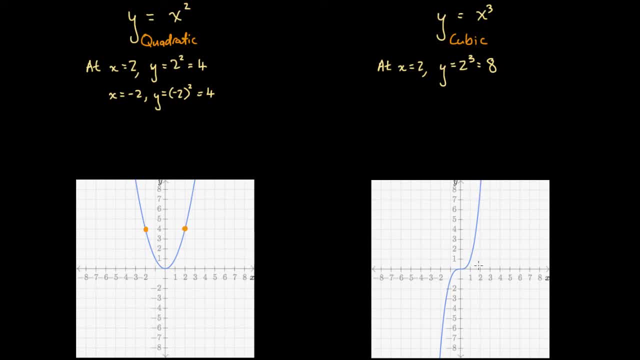 So we have x equals 2.. y equals 8.. Let's go ahead and plot that x equals 2. It's 2 units right of the origin and 8 units up, Whereas when we have x equals minus 2, we have y equals minus 2 cubed. 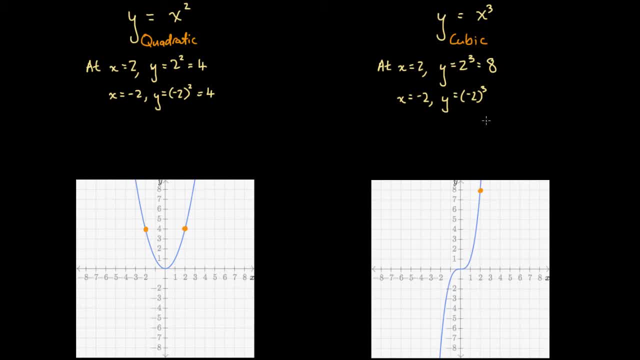 So here a negative times a negative is a positive. Then times a negative again is a negative. So this is going to be negative 2 times negative, 2 times negative. 2 equals negative 8.. Let's plot this as well. So this is 2 units left of the origin and 8 units down. 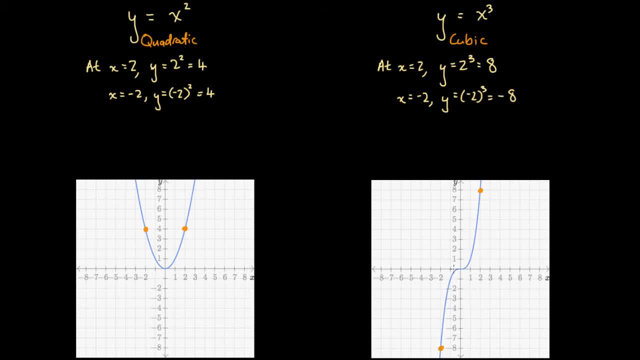 Right. So we've discovered here that the reason this left-hand side of the graph is different from this left-hand side of the graph is that when it's the property of algebraic construction, here for the quadratic function, a negative times a negative is a positive. 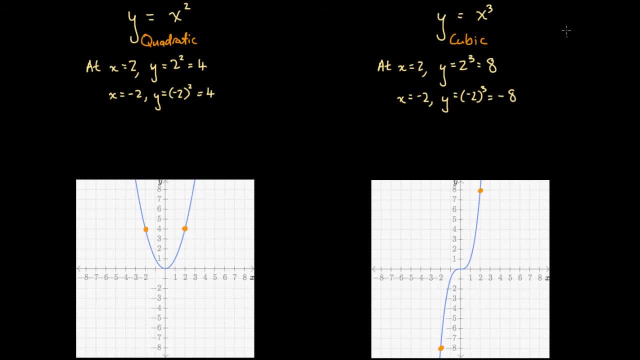 But for the cubic function a negative times, a negative times, a negative is a negative number. So that means, if we substitute a positive x value into this equation, we'll get a y value that is positive, But if we substitute a negative value, we'll get a y for x. 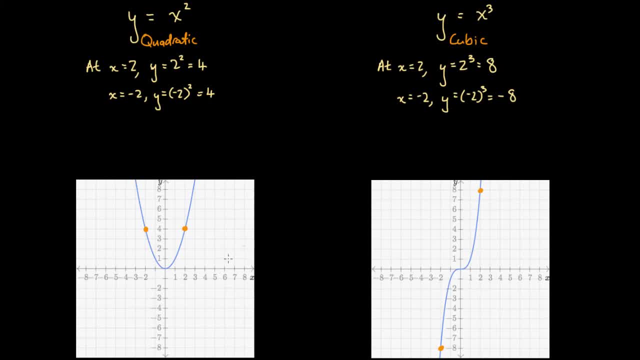 We'll get a y value that is negative. That's why these graphs look so different on the left-hand side. Okay, Well, that's interesting. Let's have a quick look at what the implications are for two important features of graphs. The first one is that x equals 2.. 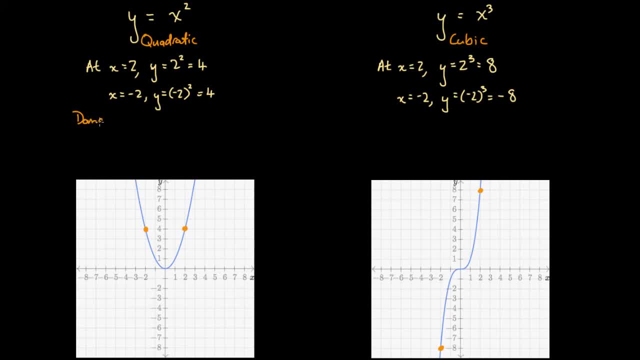 And that is, let's have a look at the domain of each graph, the range of each graph and also let's have a look at whether they are odd or even functions. So firstly, the domain. You might recall that the domain is the set of possible x values that we could input into. 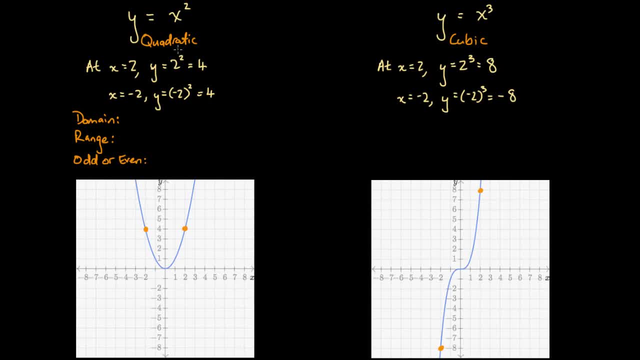 this equation. Well, for both equations we could input any x value here. There are no x values that we could that if we input them we'd get some inconsistency or some inconceivable y value on the left-hand side of this equation. 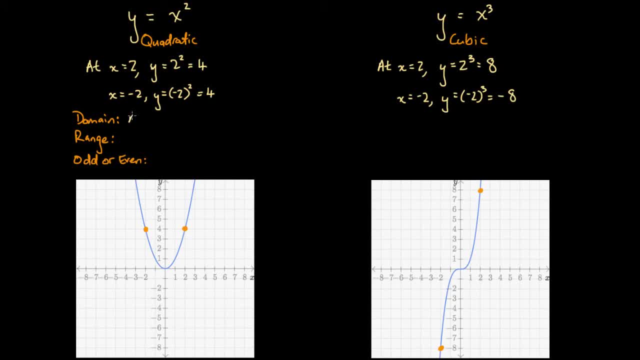 So consequently the domain for both the domain is all real x, All real x. We could substitute any real x in here. This is right Domain Range And odd. So we can substitute any real x value into either of these equations and we get a valid. 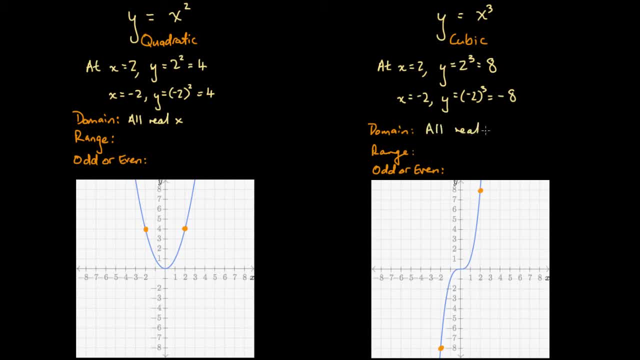 y value as an output. So consequently all real x is the domain. What about the range? Well, here we can never have a negative y value. So consequently we could never input an x value in here and retrieve a negative y value. 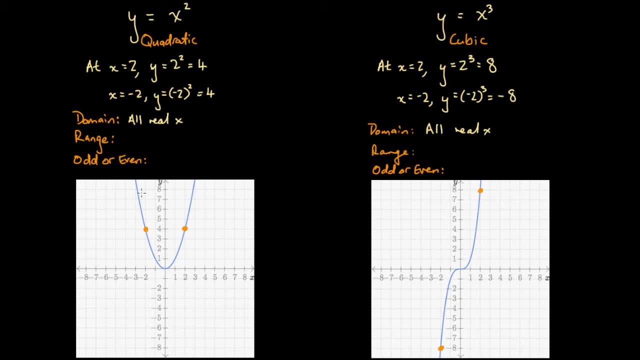 We do have y equals 0 at x equals 0. But apart from that, all the y values Are greater than 0. And they extend, you know, forever upwards, So all the way to infinity. So what we've got here is the range is going to be: y is greater than or equal to 0.. 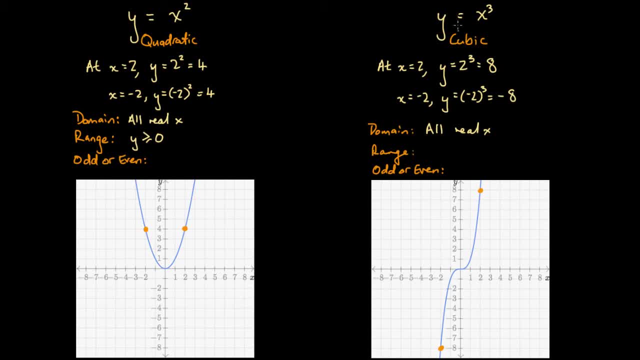 Greater or equal to 0.. Alternatively, the range here for any we can have any value of y could be output from this equation. Any negative value or positive value or 0 value of y is going to be associated with a positive or a negative or a 0 value of x. 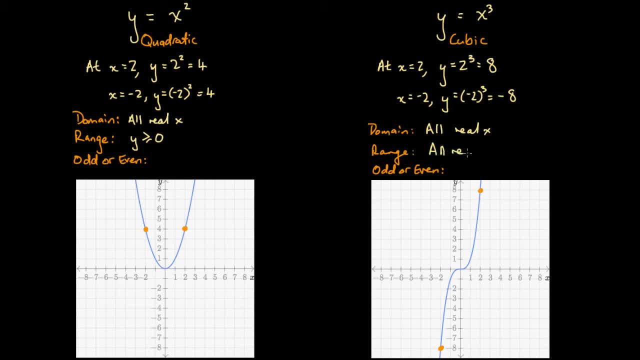 So, consequently, the range here is all real y And that's interesting that we have this different, this different, these different ranges. And again there are consequences of the property of multiplying negative numbers and whether the product of two- you know the fact that the product of two negative numbers- is a positive. 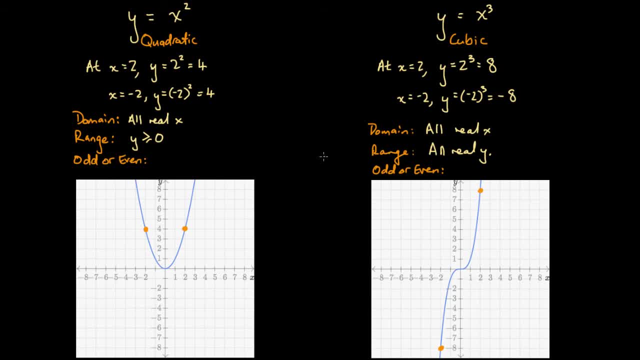 number, but the product of three negative numbers is a negative number. That's the reason we've got these different ranges. Fine, Finally, let's consider whether each of these functions is odd or even, and we could do this in two ways. 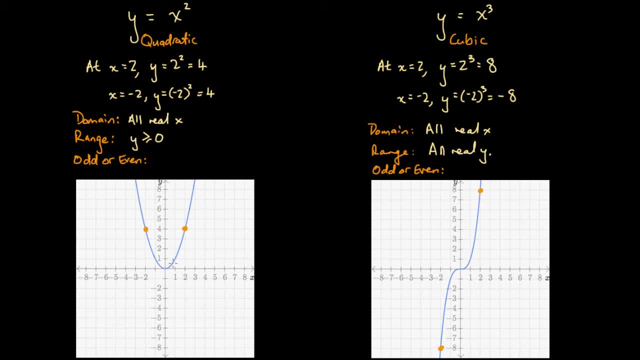 The first way we could do it is simply look at this graph and say, ah well, this graph. it has a cemetery around the y-axis. If we were to rotate this graph in the in the y-axis, or if we were to deflect it in? 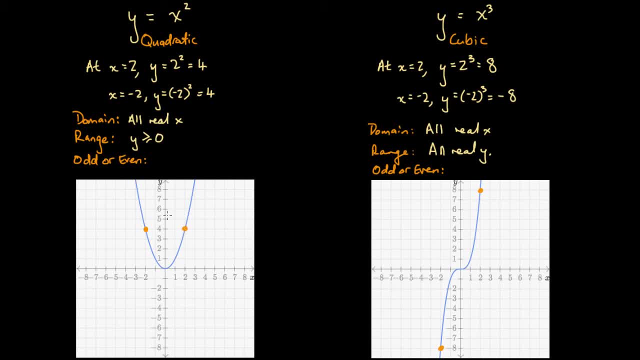 the y-axis, we'd get exactly the same graph that we started off with And consequently we could say that it is even An alternative way of finding out whether or not it's even or not. I'm going to go back to the previous slide. 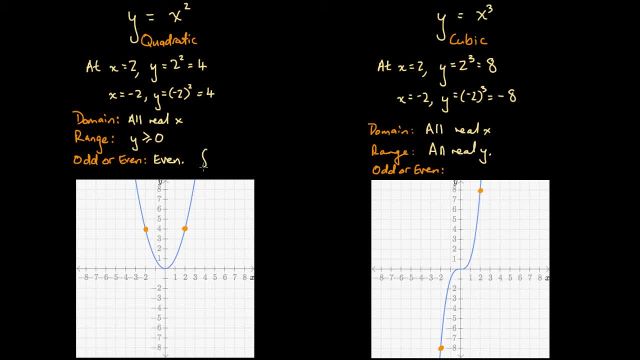 The last way. the next, the last way that you're going to find out whether or not the graph is even or odd is we could recognize that we could rewrite this function as f of x equals x squared. This captures the same idea as y equals x squared. 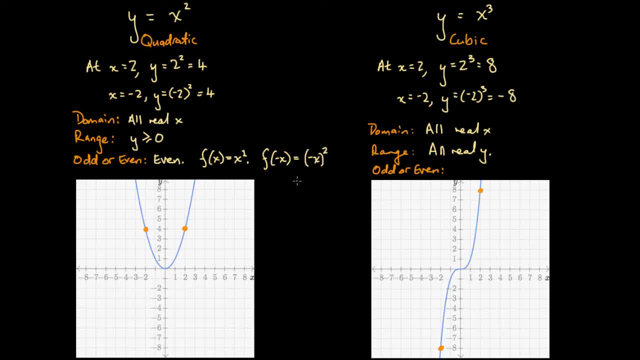 And then we could examine what happens when we substitute minus x in this equation. So let's evaluate f of negative x. So here we'd get negative x squared, Negative negative x squared, And negative x squared is x times x is x squared. 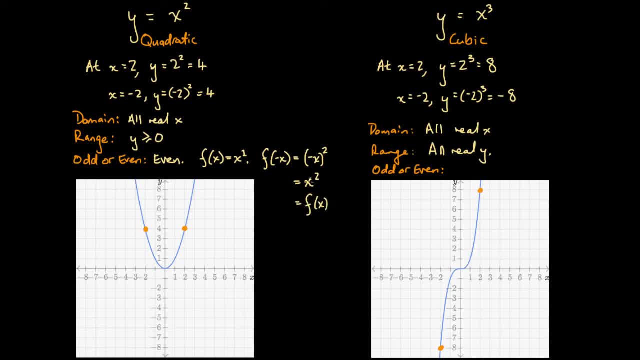 Negative times a negative is a positive. so this is x squared. Okay, Well, this is the same as our original fx, because x squared equals fx. So here we have f negative, x equals fx and this, this is the definition of an even function. 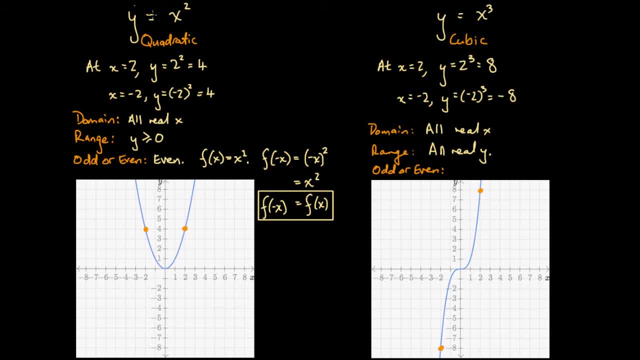 All even functions have this property. So, consequently, we can say that y equals x. squared is an even function. Well, what about y equals x cubed? Again, we could consider this both graphically and algebraically. Well, graphically, we can see that this function has point symmetry around the origin. 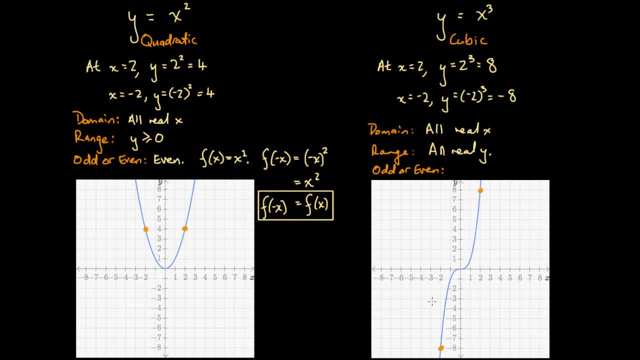 So if we were to rotate this graph around the origin 180 degrees, we would get exactly the same graph as we started. So we could say that this. we could say here that this graph is odd. Alternatively, if we wanted to figure this out, we could recognize that y equals x cubed.